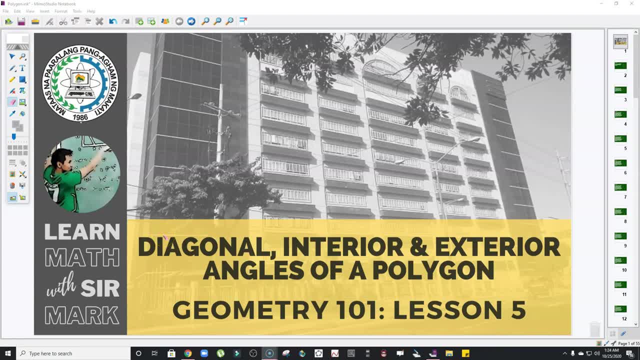 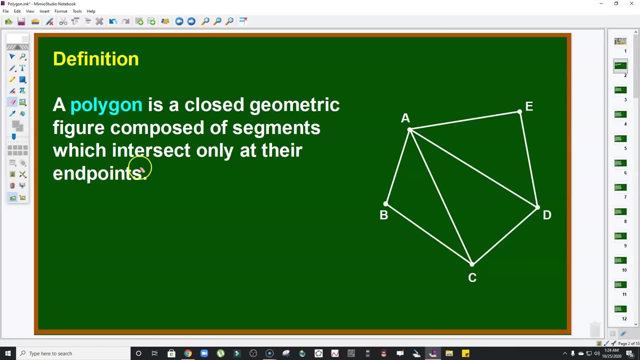 let's begin. Okay, first let us define what is a polygon. A polygon is a closed geometric figure composed of segments which intersect only at their endpoints. The segments are the sides of the polygon and the intersection of the endpoints are the vertices. Any segment 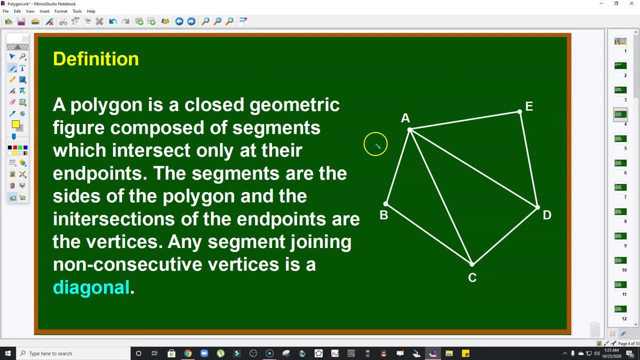 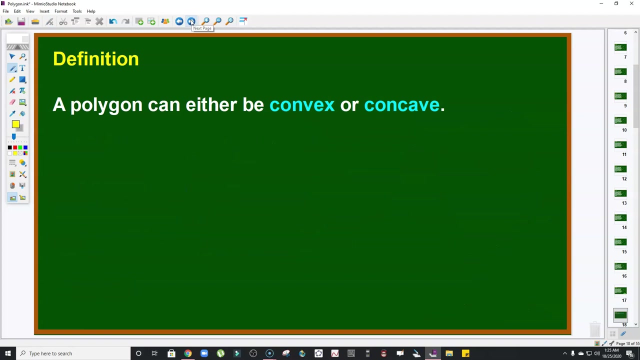 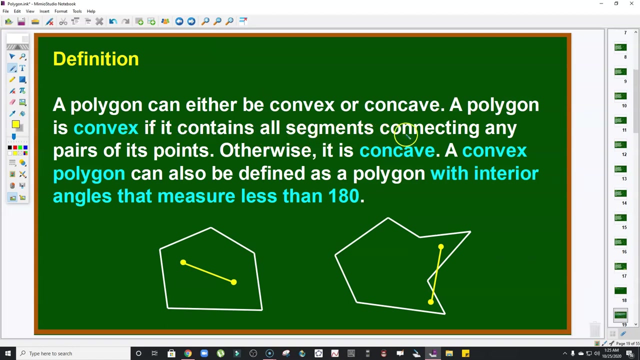 joining non-consecutive vertices is a diagonal. So in this given illustration, the segments AB, BC, CD, DE and AE are sides of the given polygon, while the points A, B, C, D and E are the vertices. Now let's look at examples of diagonals Next, a polygon can either be convex or concave. We said a polygon is convex if it contains all segments connecting any pair of its points. Otherwise it is concave, As you can see on the second figure. this is an example of concave because, as you can see here, it's not included in the polygon. 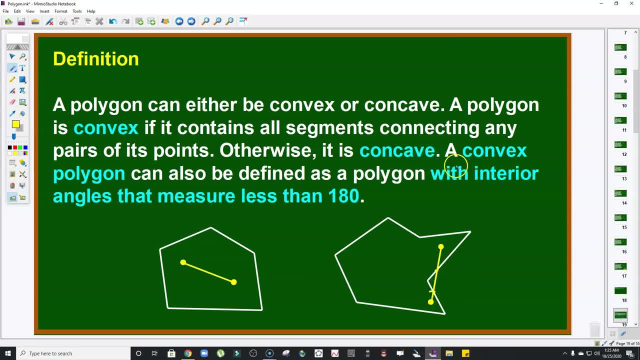 These are the points. See that, Okay. Next, another definition is that a convex polygon can also be defined as a polygon with interior angle that measures less than 180.. Once again, the first one is convex, The second one is concave. Okay, I'd like to emphasize here: this is obviously greater than 180, thus making it. 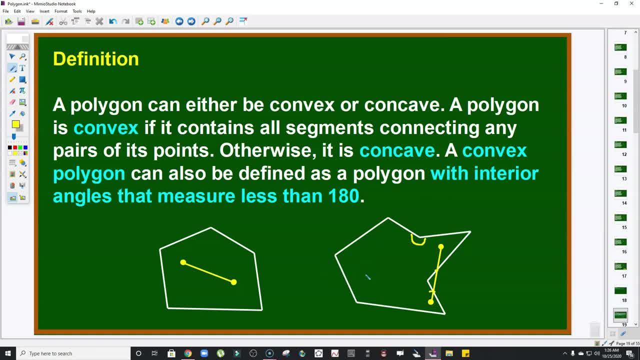 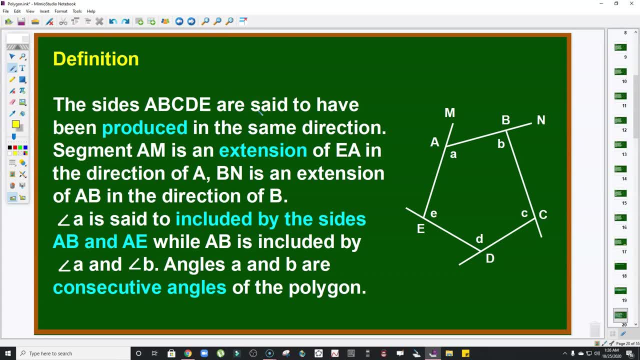 concave. Okay, Next, the sides A, B, C, D, E. The sides of A, B, C, D, E are said to have been produced in the same direction. Okay, Segment AM. this one is an extension of EA in the direction of A. Okay, starting from E towards A. so this is: 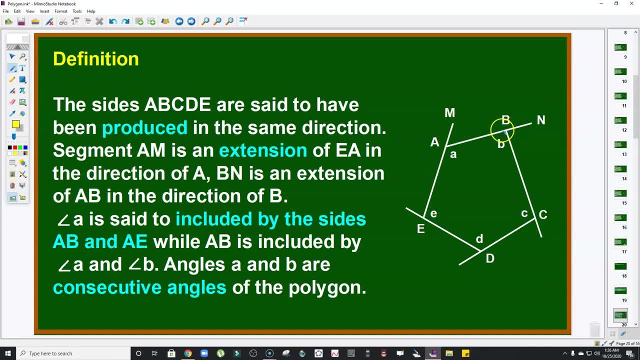 the extension, while BN is the extension of AB in the direction of B, So angle A, this one, angle A, is said to be included in the direction of AB, So angle A is said to be included in the direction of AB, So angle A is said to be included in the direction of AB. 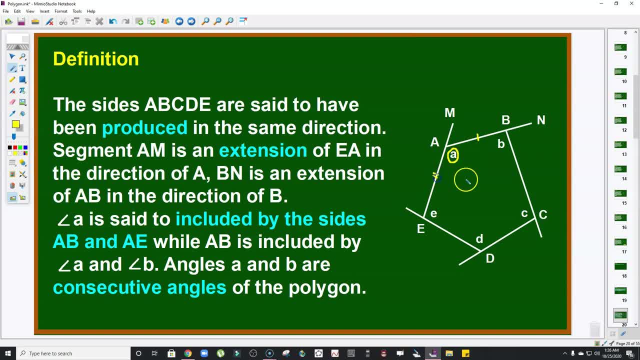 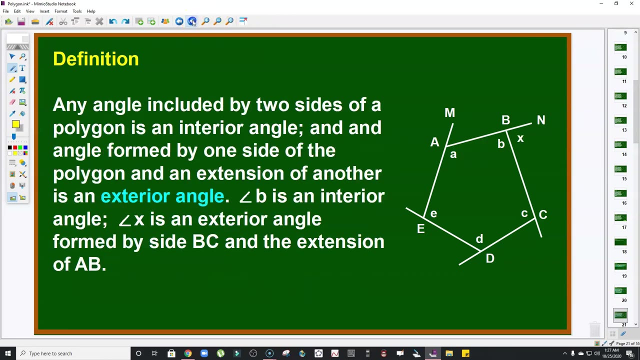 So angle AB is included by the sides AB and AE. See that, While AB is the included angle, included side by angles A and angle B. See that, Okay, Angles A and B are an example of consecutive angles of the polygon. Okay, Next, any angle included by two sides of a polygon is an interior. 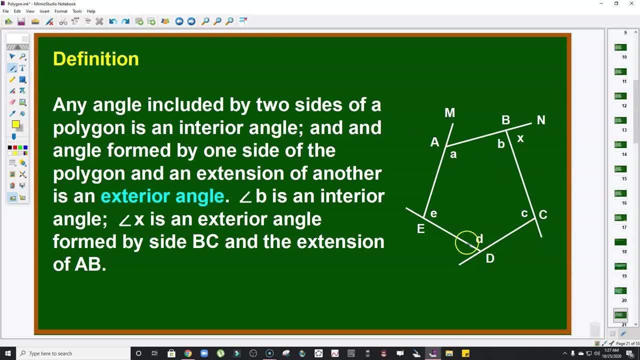 angles. as you can see here, the interior angles are angles a, b, c, d, e, and an angle formed by one side of the polygon and an extension of another is an exterior angle. so, as you can see here, this is one interior angle. this angle is made by the extension. okay, so we call this angle x as the. 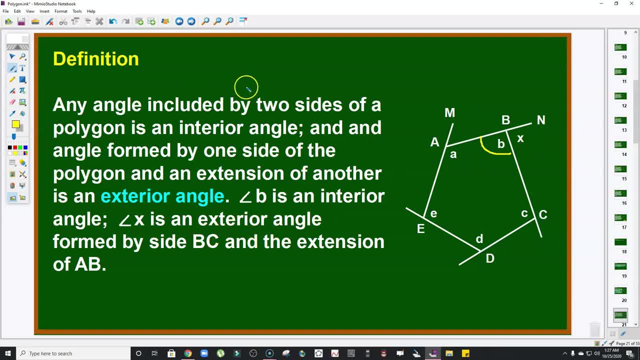 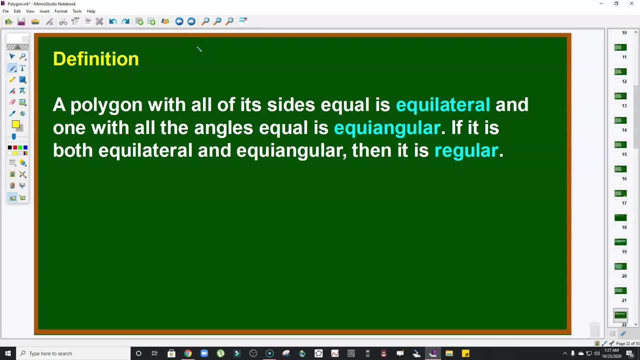 exterior angle. okay, there you go. next, another definition. so a polygon with all of its sides equal is equilateral, okay, and one with all the angles equal is equiangular. if it so happened that both equilateral and equiangular, then we said that the polygon is regular. okay now. 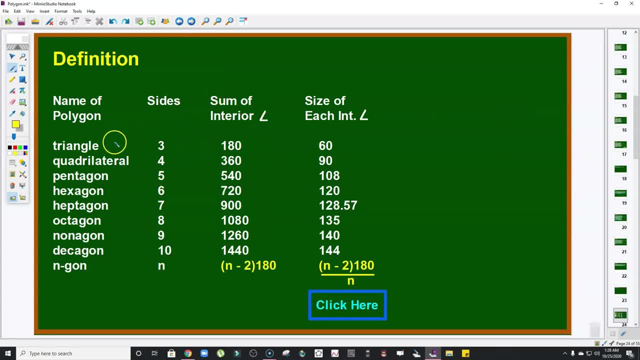 here are examples of the polygons with their names. okay, so with the given sides, and then the given interior sum of interior angles. okay, and then this is. this table here refers to the measure of each interior angle of a regular polygon. so once again, to get the sum of interior angle. so the formula is n minus 2. 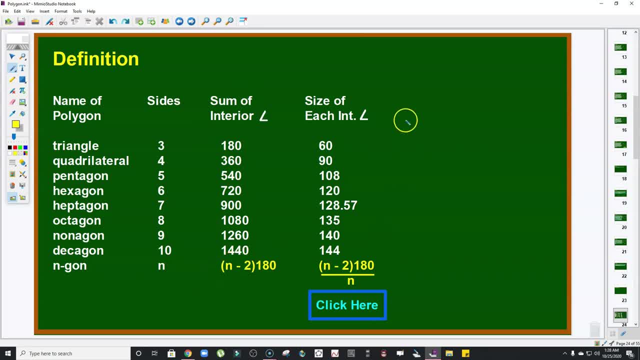 times 180. see that, on the other hand, if the polygon is given, and that is regular, okay, for after, for the, the measure of each interior angle of a regular polygon, we use this formula: n minus 2 times 180 over n. now let's take a look at this. okay, as you can see here, 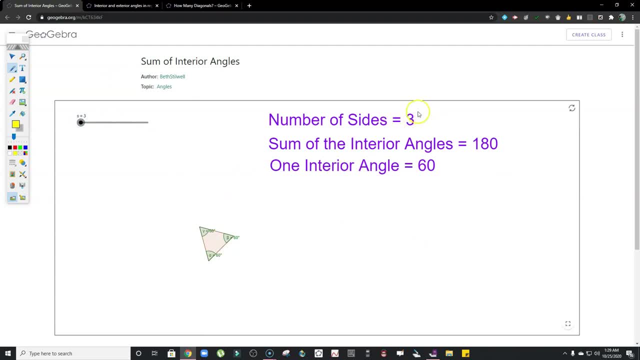 all right. so observe that this is a triangle. the number of sides is 3, the sum of interior angles 180, and we all know that, and one interior angle is 60. so regular. yeah, now look what will happen if square. okay, so it's already varying. so the interior angle is nice, so the value is zero. 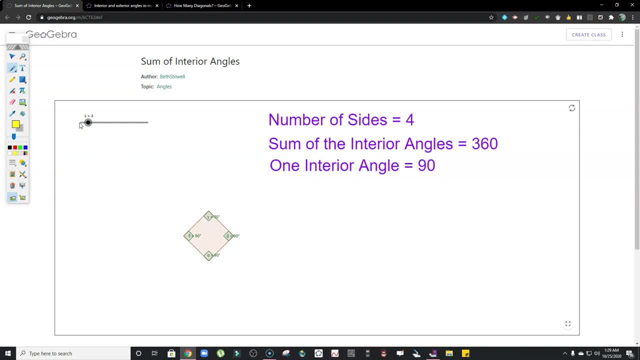 sketch and we want that to draw an estimate of 0. so we draw and transform it using this value. we also make sure that that area also can grow into theelia itself. okay, so we then have a normal. Now look what will happen if square. okay, so it's varying now. so the interior angle is 90 degrees. 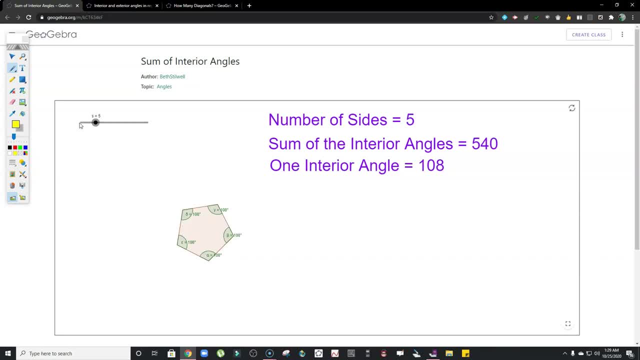 angle is 90,, okay, kapag pentagon. so the interior angle is 108, the sum is 540, and so on. See that Okay. so until we have the andekagon and dodecagon. See that Okay. 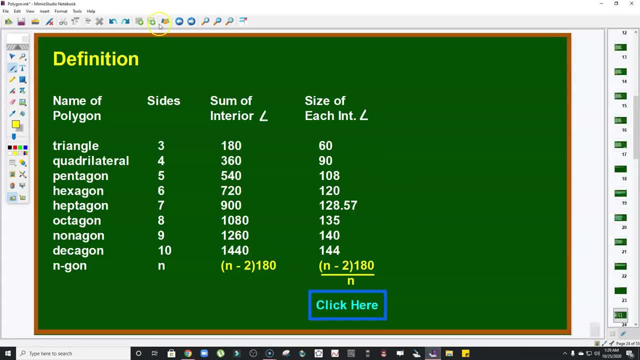 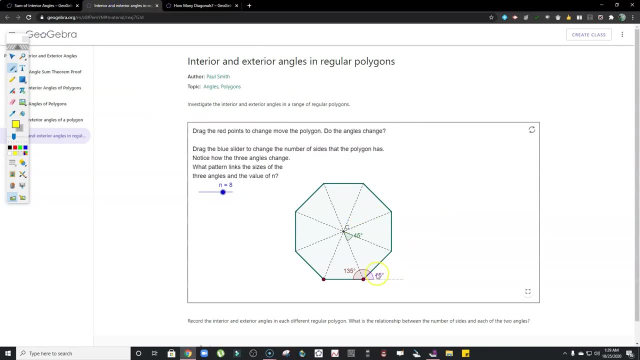 Okay, Next, Okay, The sum of the exterior angle is always 360.. Okay, I'll show that. Okay, pakitan natin. Okay, so this is an exterior angle, yung 45, okay, So magstart tayo dito. Alright, so the 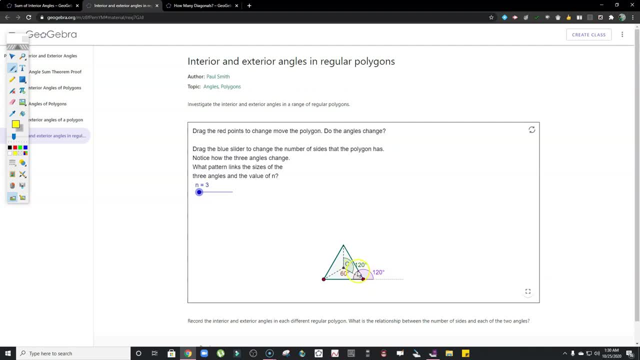 exterior angle here is 120.. Alright, so the interior angle here is 60.. So together they form a linear pair. So that's why the sum is 180.. Now look what will happen. Okay, kapag kwadrilateral, we have this pentagon, hexagon. 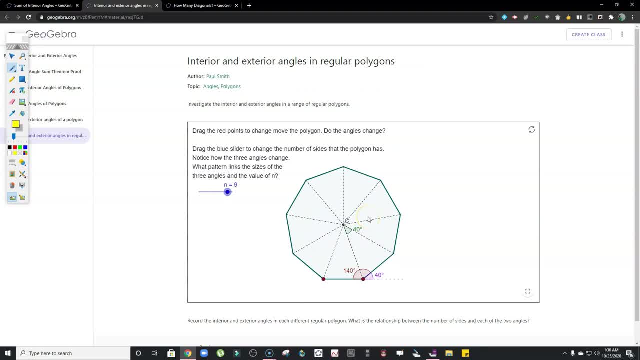 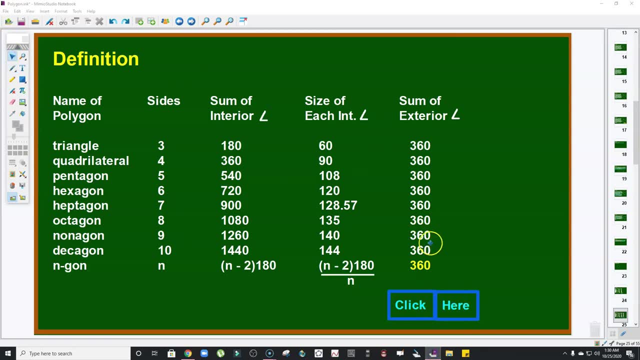 two-fourths: heptagon, octagon and nonagon, dodecagon. So there you go, See the relation. Okay, now let's add this. Now, like I said, pakitan natin bakit 360?? 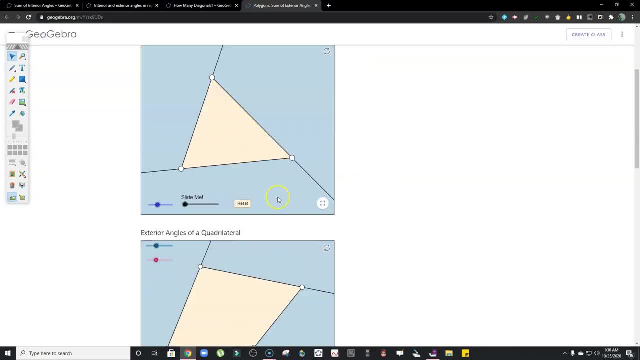 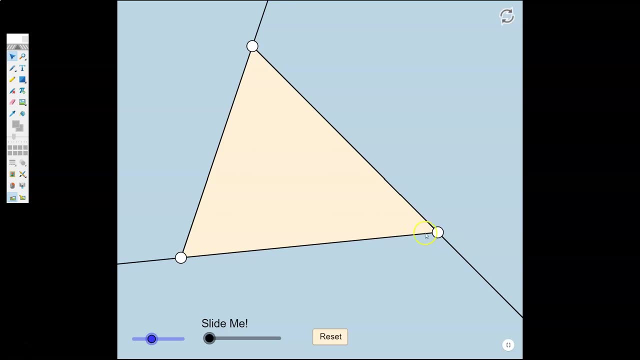 Okay. so, as you can see here, this is an example. okay, This will show you that the sum of the triangle, the angles of the exterior angle, the sum of the exterior angle is 360.. So look at this, Alright. so this, okay, look at this. So yung red na yan, okay, is an example of exterior angle. right Now, this is the second exterior angle. Now look what will happen. 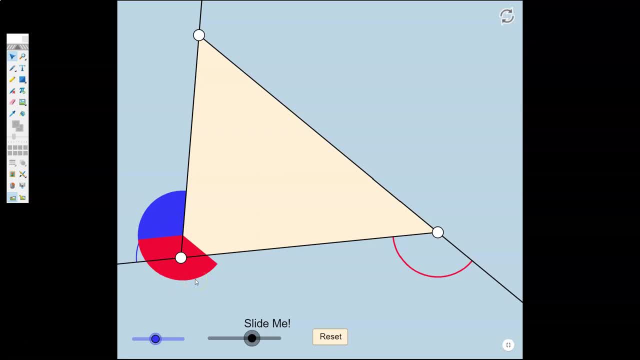 Okay, yung red and then yung color blue. okay, Okay, yun yung sum nila. Then this is the third one, As you can see here. okay, that completes one revolution, So that's why the sum is 360.. 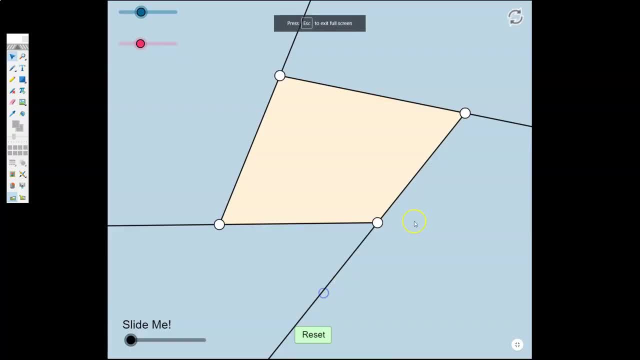 See that? Okay, now tingnan natin kung kwadrilateral. Okay, tingnan natin dito. Alright, so same This green here, yung blue, yung red na exterior angle and last yung purple, So together 360.. 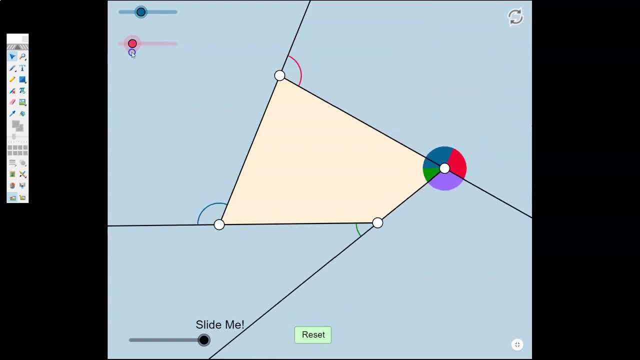 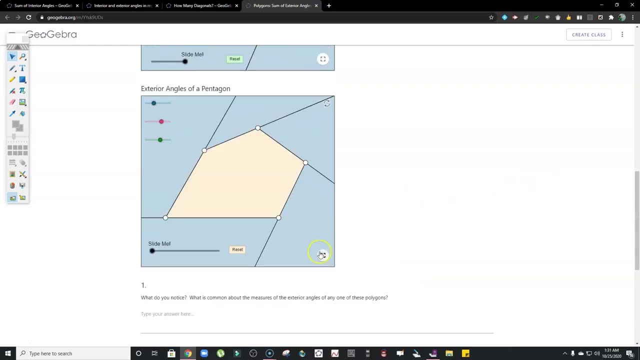 Kahit baguin ko yung size ng kwadrilateral ko, still the sum of this exterior angle, this, this and this is always 360.. See that? Okay, let's change that, Alright. Okay, now let's look at the pentagon. 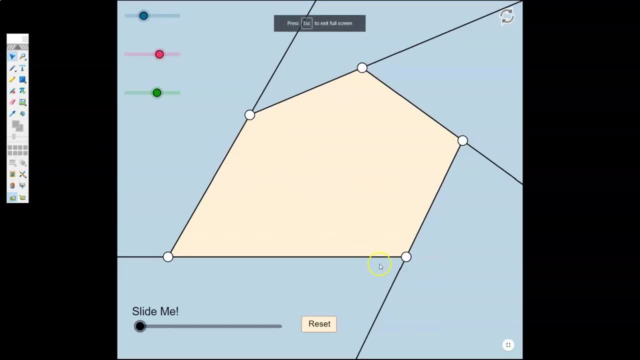 Okay, so one more Pentagon again. so look at this. So this one, the orange one, is an exterior angle, Right? Okay, as well as this, There, that's an exterior angle, and so on. 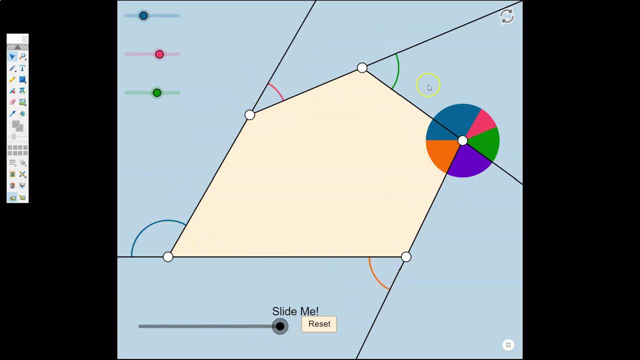 There you go, So 360, again: itong orange, itong blue, itong pink, itong green, and this one, the violet, one 360. kapag in-add mo Again, kahit baguhin mo yan, okay, still hindi magbabago yung sum ng exterior angle. 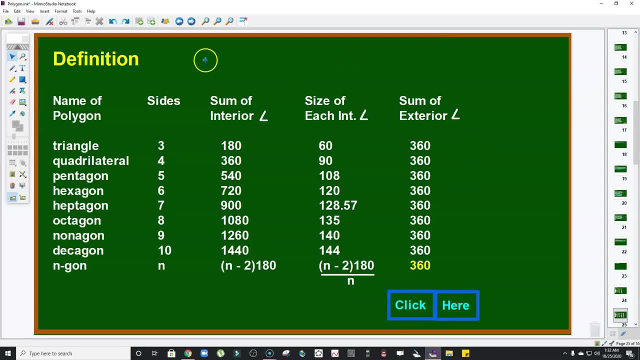 See that, Okay. Next, So the measure of each exterior of a regular n-gon is 360 over n. Okay, we know that. Next, Lastly, Okay so the number of diagonals. okay, here are the table with the kung triangle: no diagonals. kung quadrilateral: two diagonals, and so on. 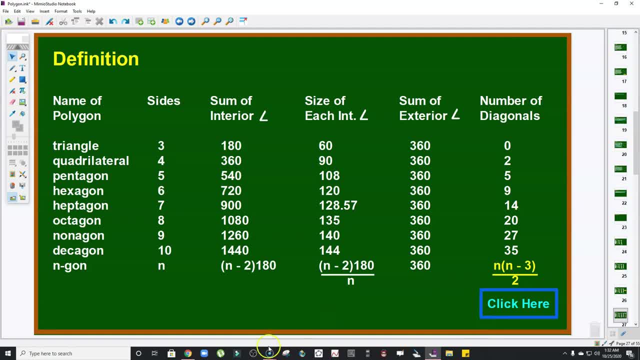 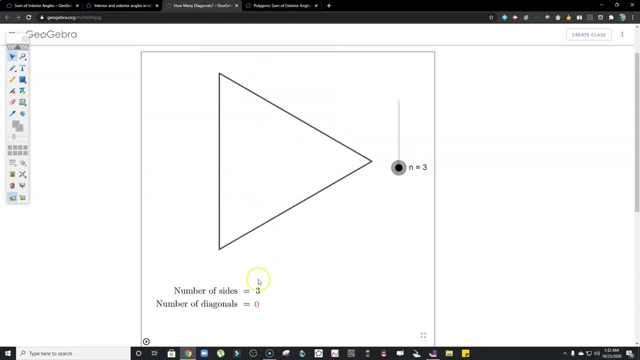 So the formula there is n times n minus 3 over 2.. Okay, So that is where's that? Okay, this one, As you can see here. number of sides: 3, that's triangle. Number of diagonals: none. 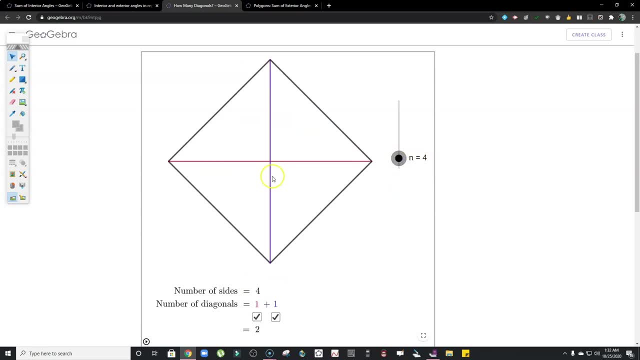 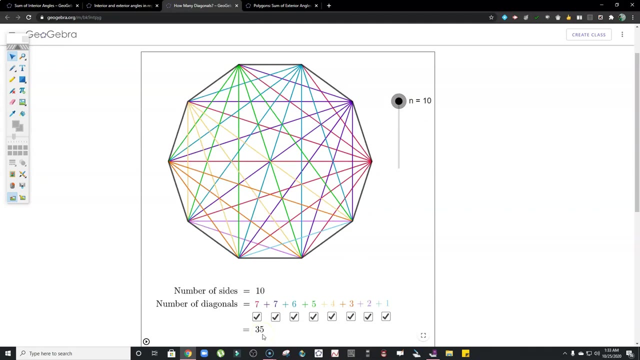 So now look what will happen kapag quadrilateral. so obviously there are two diagonals. Okay, when we have a pentagon we have five diagonals: hexagon 9, heptagon 14,, octagon 20,, nonagon 27,, decagon 35.. 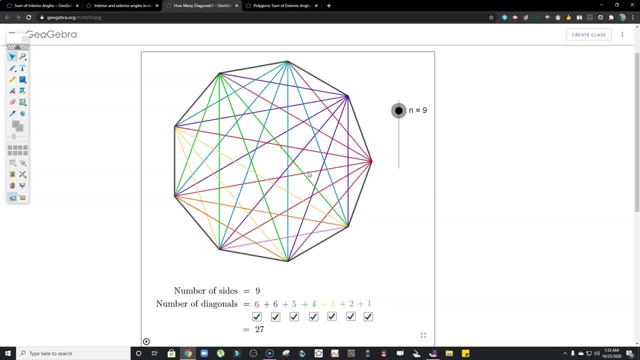 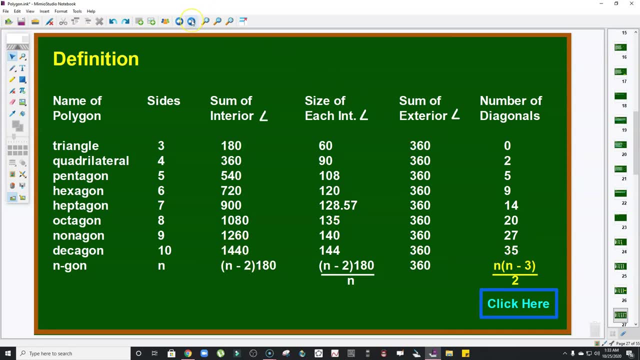 There you go. Amazing, right, Cool. Okay, now let's go back. So that's it. Once again, take note of the formula: Okay, we'll apply that later. Okay, now let's start. example number one: 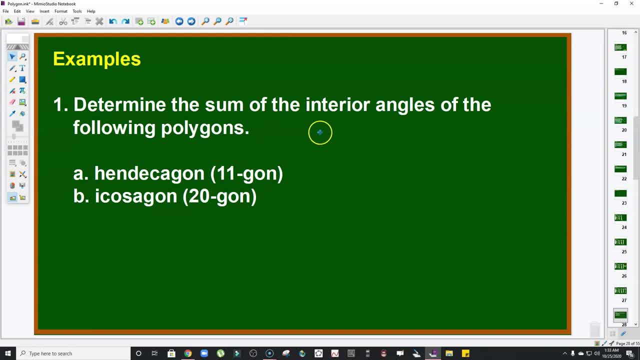 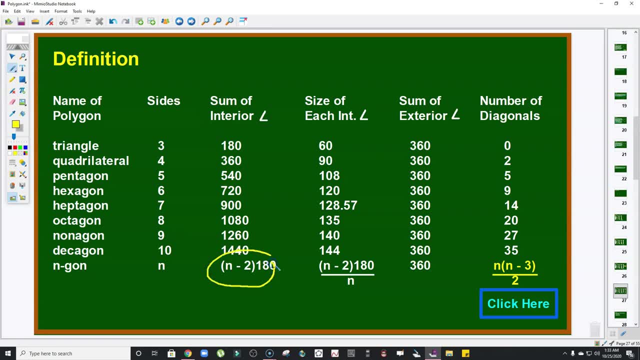 Okay, now let's start. example number one: Determine the sum of the interior, The interior angles, of the following polygon. Once again, the formula kapag interior angles, sum of interior angles is n minus 2 times 180.. Okay, let's have number one. 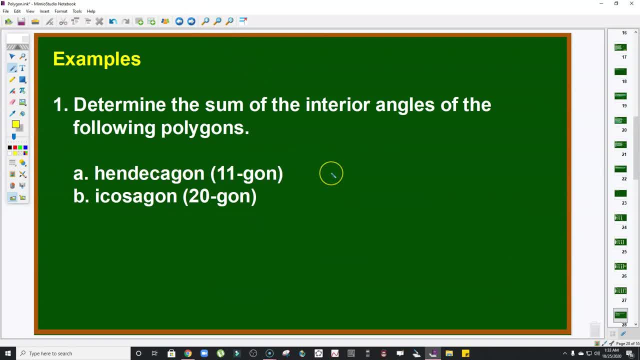 Okay, this is just a special name: Hemdecagon, that's 11 gon, So meaning to say once again n minus 2 times 180.. Ito lang yung gagamitin natin formula. So that is for letter A, so we have 9 times 180.. 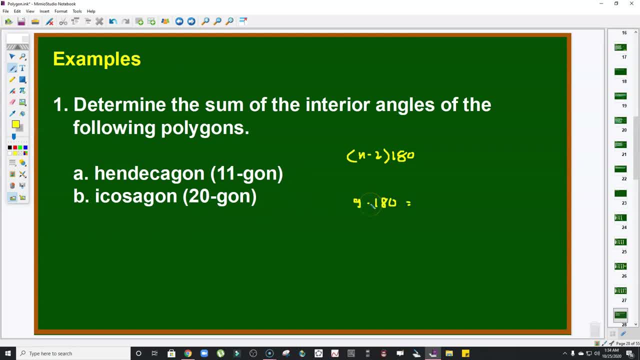 As simple as that. Okay, so that is 9 times 180.. So that is 1,620.. Clear, Okay, that's for letter A. How about for letter B? So icosagon, that's a polygon with 20 sides, or 20 gon. 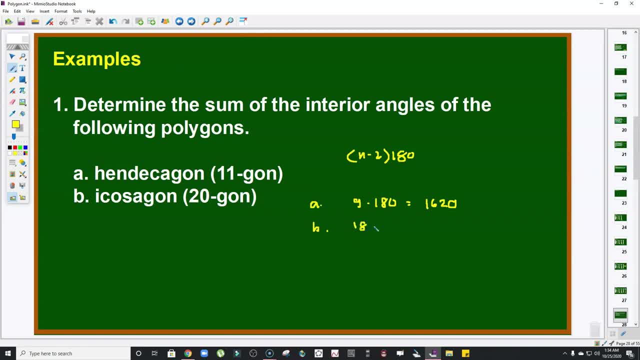 So meaning 20 minus 2.. So that's simply 18 times 180.. And we know, okay, 18 squared that is 324.. Right Times 10.. So that's why 3,240.. 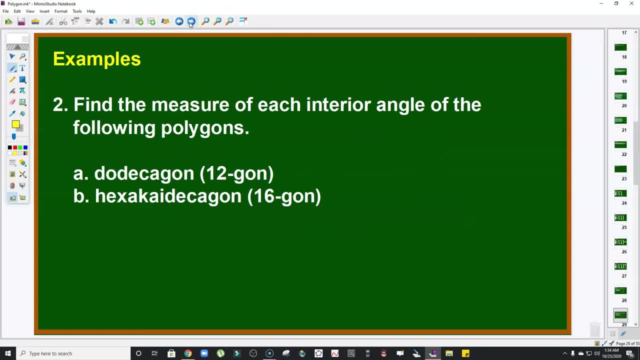 Simple right. So once again, don't forget the formula Next, number 2.. Find the measure of each interior angle of the following polygons: Okay, for the decagon measure of each interior angle of the regular polygon to. 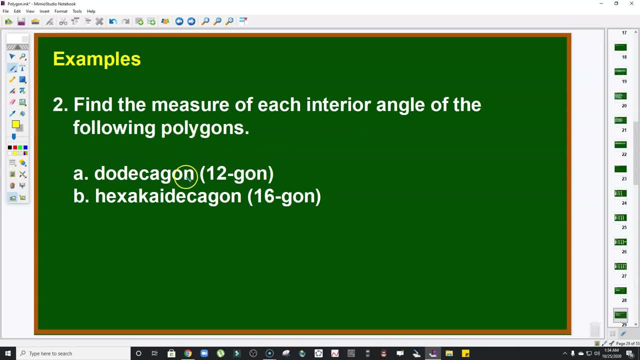 Regular, Okay. so Now kapag the decagon, so again yung formula: kapag regular polygon, interior angle, So that's n minus 2. So that's n times 180 over n okay. So that's why for letter A: 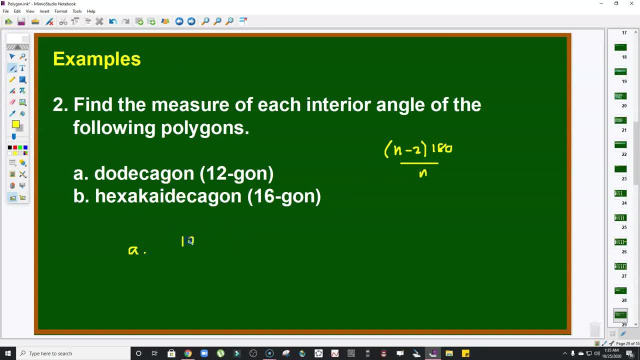 So since 12 sides yan, so we're going to have 12 minus 2, that's 10 times 180 over 12.. Okay, so let's simplify. So this 12 here is 4 times 3, okay. 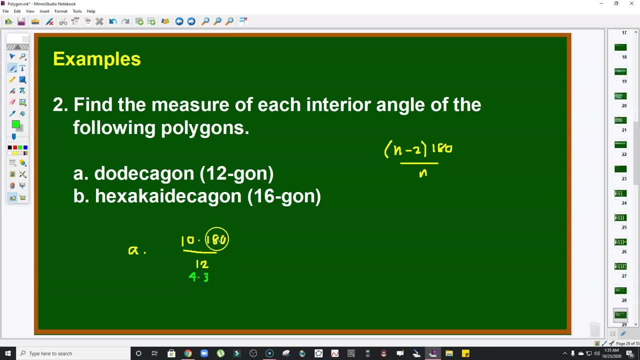 4 times 3 yan. Well, this one here 180,. that is 4. 145 times 4, right, Or 15 times 3 times 4.. Clear, Okay, so clearly maka-cancel ko ngayon tong 4 and 3.. 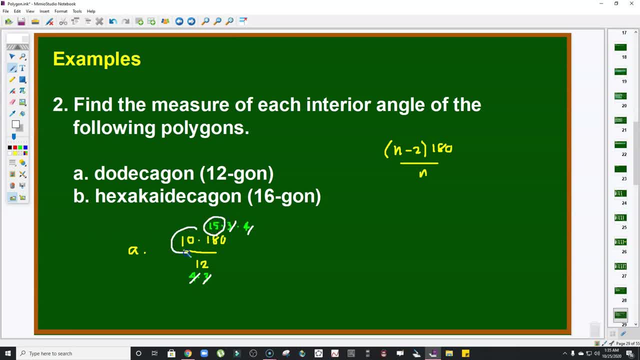 Okay, So what will be left here is just 15 and 10.. See that. So, therefore, each angle of a regular decagon is simply 150.. See that, Okay for letter B: hexa-kai-decagon. 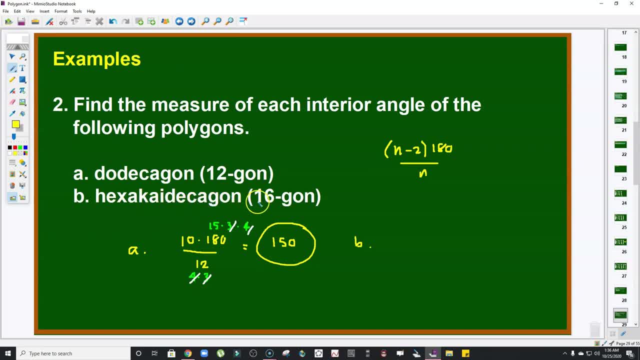 Again, you don't need to memorize this, pero, just for the information. okay, So that's it, Kung 16 gone. so that is 16 minus 2, that's 14 times 180 over 16.. 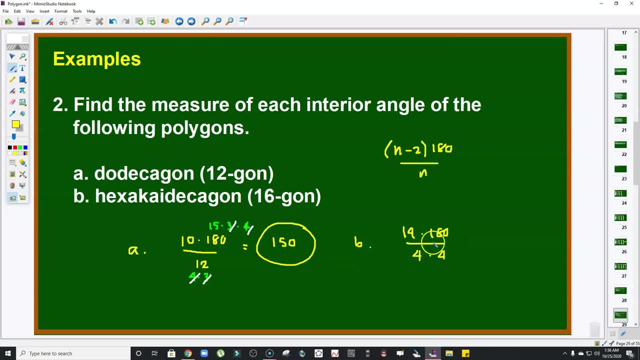 And 16,, that's 4 times 4.. Okay, again I did like it, I did it parang ganito. okay. So ang 180, again nakita ko na yan kanina, So that's simply 45.. 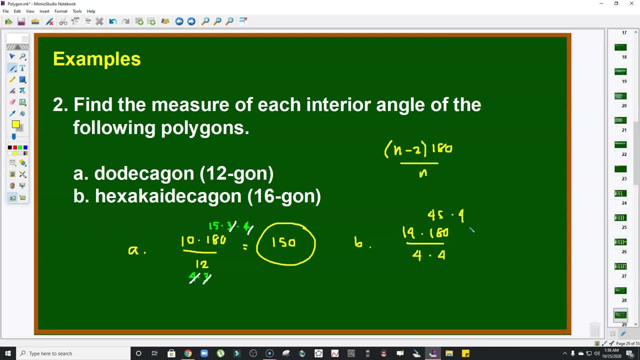 45 times 4, right Now tapos yung set 14, that's 7 times 2.. Okay, so that maka-cancel ngayon tong 4.. Okay, maka-cancel ngayon tong 2.. 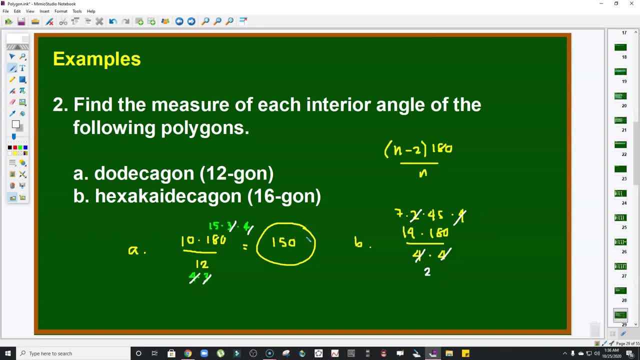 Okay, so fraction yan. So 7 times 45.. Okay, so that is 315.. Okay, I'll use yellow. Okay. Okay, That's okay: 245, that's 315 all over 2.. 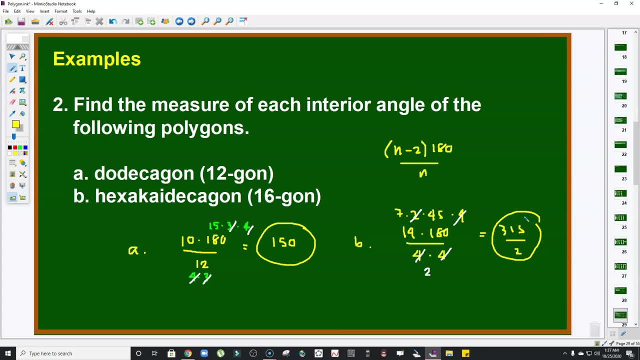 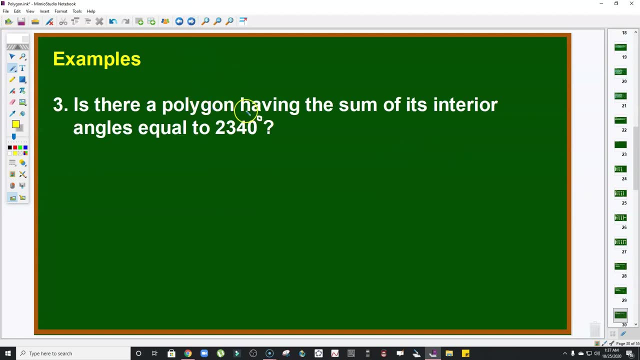 Alright, So or gawin nyo na lang: ano 315 over 2 or 157.5 degrees. There you go, Okay. next number 3.. Is there a polygon having the sum of its interior angle equal to 2340?? 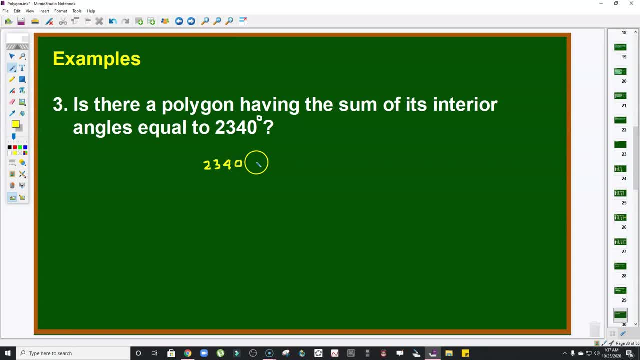 Okay, let's find out. So 2340,? okay, Ang tanong meron bang polygon Sum is like that. So syempre equate natin sa formula na n minus 2 times 180.. That is so n minus 2.. 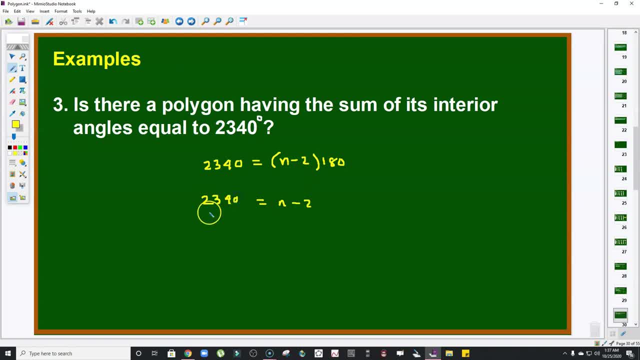 So what I'm going to do is to divide 2340, okay, by 180.. Okay, cancel yung 0 o yung 10.. Okay, 234,. nakita natin yan, kanina. 234 divided by 18, that's 13,, right. 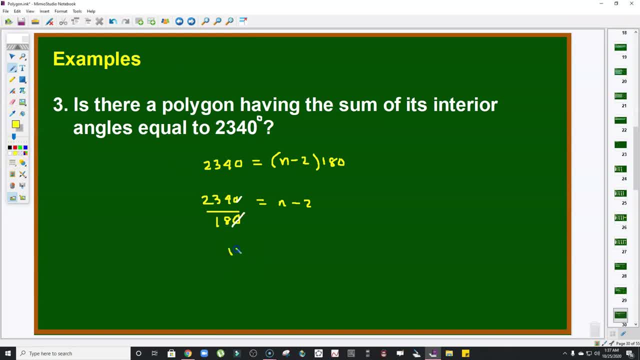 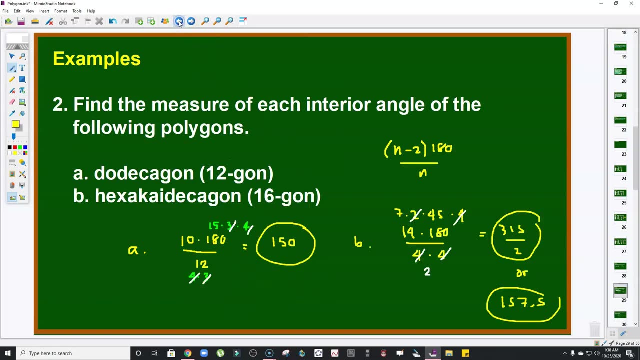 So that's 13.. Okay, equals n minus 2. So clearly n is 15.. So therefore, the question: is there a polygon? Yes, And that is pentadecagon. Okay, pentadecagon nga ba yung 15?. 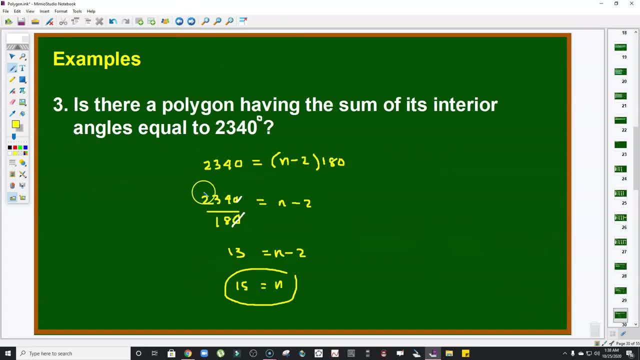 Ah, wala, Anyway, huwag tayo mag-ibeta na. nun, It's just 15 guns, okay. Next number 4.. How many triangles are formed when diagonals are drawn from One vertex only of a hektagon? 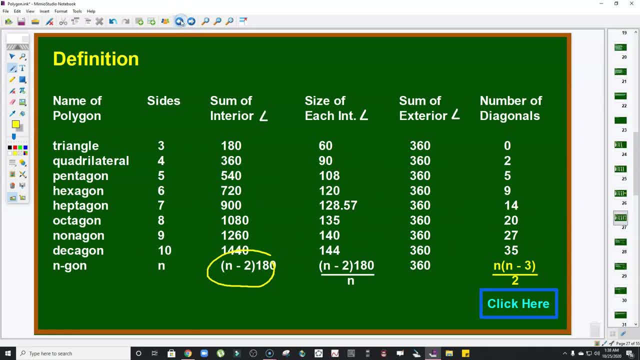 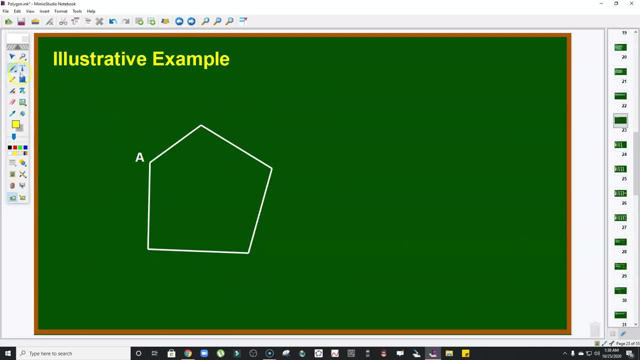 Okay, ito yung binigay kong activity sa inyo guys. Okay so balikan natin ito. ah, okay, So in your activity. so, diba, if you remember from one vertex, okay, so you're going to. 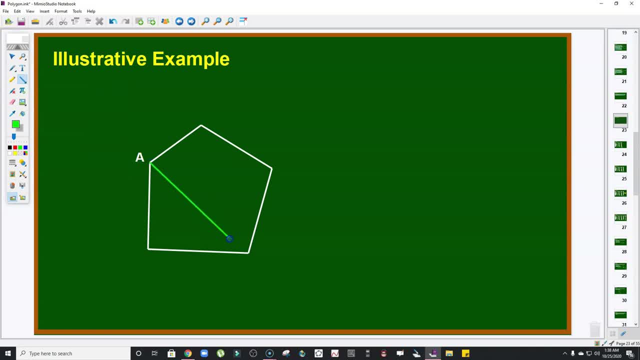 connect it to the other. ah, connect ka ng diagonal, tama, Okay. so from there kita natin how many triangles yun na form, Isa Dalawa Tatlo. So meaning, kapag five sides, okay, kapag five sides, so five sides, so you're going. 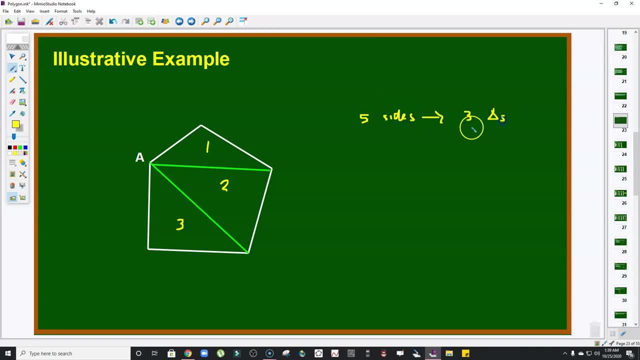 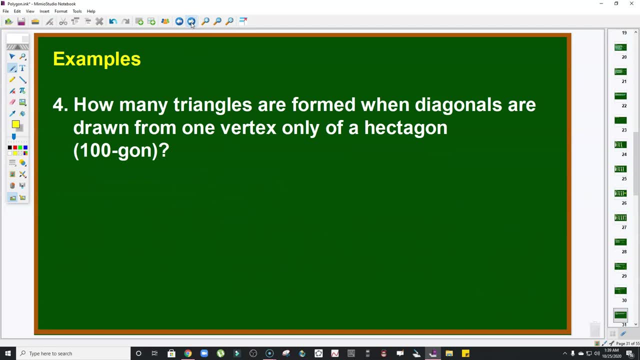 to form, ah, three triangles, So minus 2 lagi. Okay. So nakita nyo yun dito right nung pinil up nyo yung activity. So meaning to say so ang tanong: how many diagonals okay, kung 100 gun drawing from? 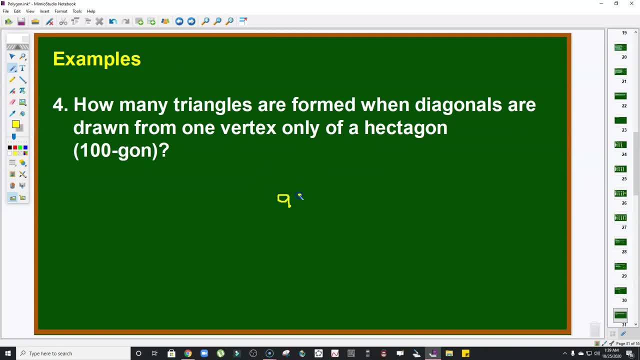 one vertex only. So the answer here is just 98. Okay, 98. Clear. Next number 15, what is the sum of the exterior angles of a pentadecagon? Okay, Sum of the exterior angles. So binigay ko na yun. 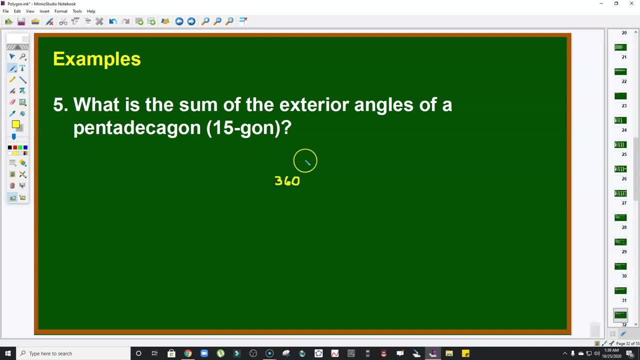 So automatic yun. ang sum ng exterior angles of any n-gon is 360.. Okay, And pinakita ko yun kanina Clear Next Six. If the total number of interior angles of a polygon is 60,, how many sides does the polygon? 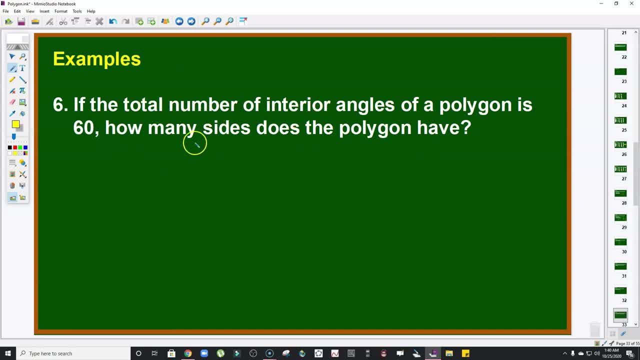 have. Take note: total number of interior angles is 60,. how many sides does the polygon have? The answer is also 60.. Kunyari triangle, diba. So I have three angles. how many sides Tatlo? 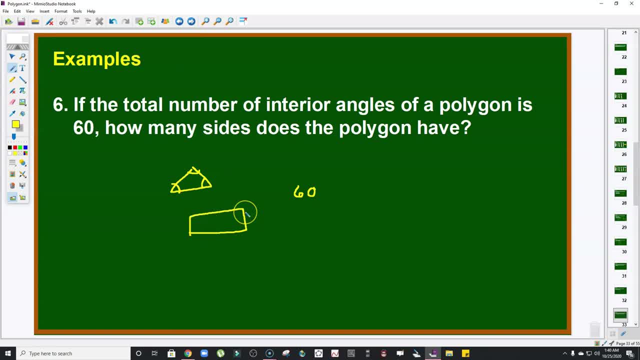 If I have a quadrilateral, I have four sides, I have four angles, and so on. So ganun lang lang, Okay. So 60 yung sagot, Okay. Number seven Determine the number of diagonals of a 14-gon. 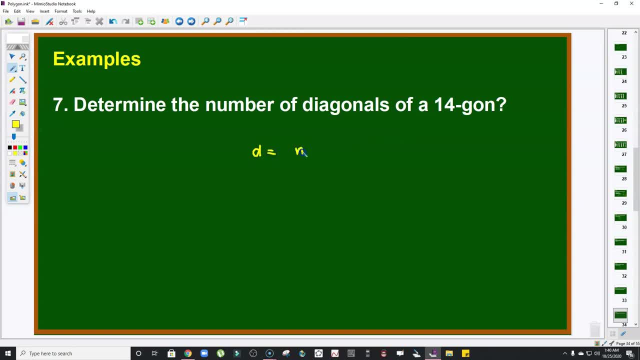 Okay, Take note ang formula for diagonals once again: n times n minus 3 over 2.. Okay, So if you're after for the number of diagonals, n is 14, so that's simply 14 times 14 minus. 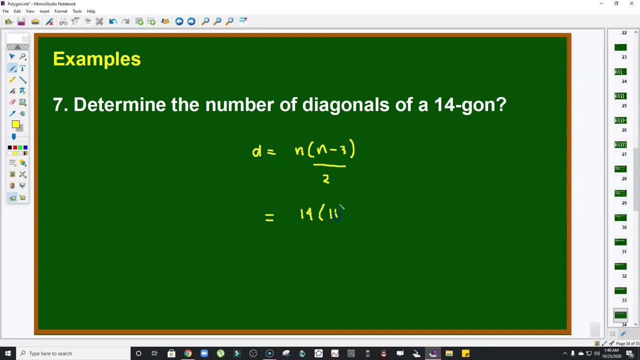 3. Tama, That's 11.. Okay, Over 2.. So clearly cancel to So 14.. So this one will become 7.. Therefore, there are how many diagonals 7 times 11.. 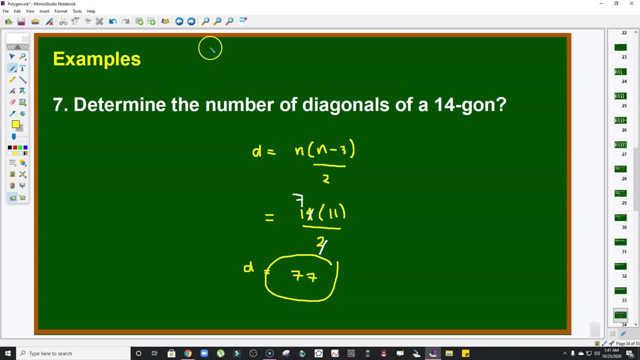 So 77 diagonals, Okay. Kapag 14-gon, Next number eight, Determine the number of sides of a polygon with 54 diagonals. So this time we're looking for n, given ang D, Okay. 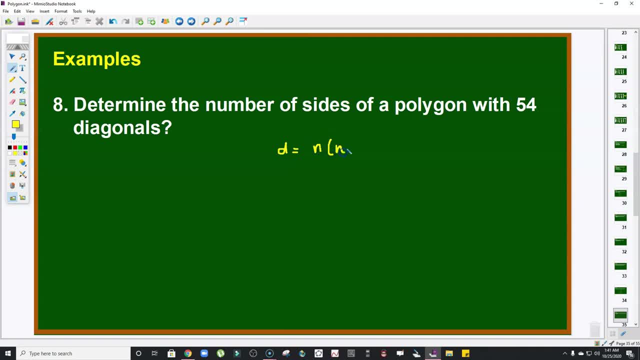 Balikan natin yung formula. The diagonal is given by n times n minus 3 over 2.. However, given to 54, we're looking for n, Tama. Okay, So cross multiply. I'm going to have 108 equals n squared minus 3n. 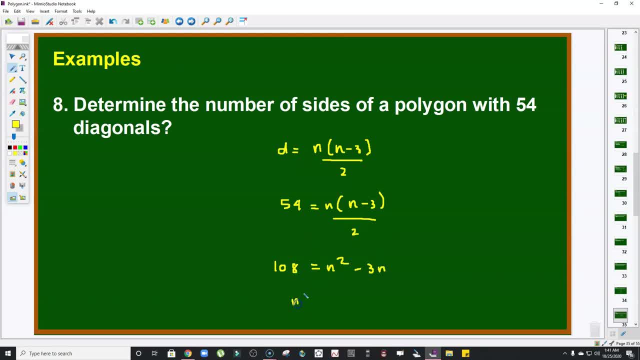 So marunong na kayong mag-factor ng ganito right In your basic math. So n squared minus 3n minus 108 equals 0.. Now factors of 108.. Okay, Ano bang factors ng 108?. 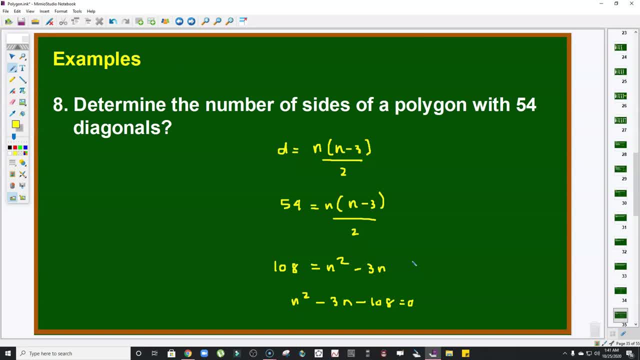 Okay, So 1 minus 3, negative 108, negative 108.. Okay, There you go. So 12 and negative 9, right? So if we're going to factor it, that's n minus 12 times n plus 9 equals 0.. 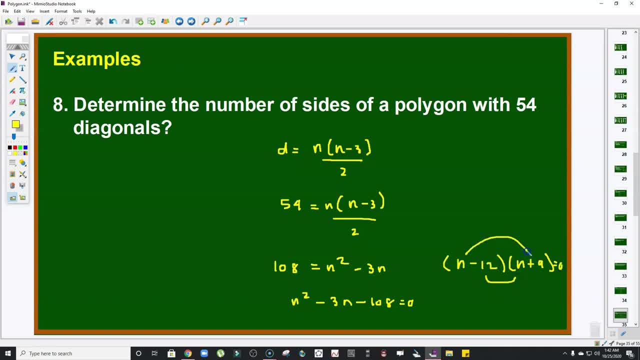 Check natin. Okay. So this is negative 12 and this is positive 3n. Negative 3n nga naman Okay, Therefore, so n is 12.. We reject n equals negative 9.. Alright, So since we're looking for sides, bawal maging negative. 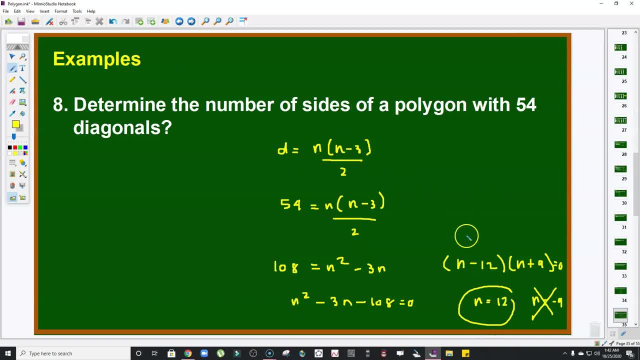 So therefore, this is: n is equal to 12 or the decade 1.. Clear Next number: 9.. Find the ratio of the angles of a quadrilateral. Okay, The ratio of the angles of a quadrilateral is 1 is to 2, is to 3 is to 4.. 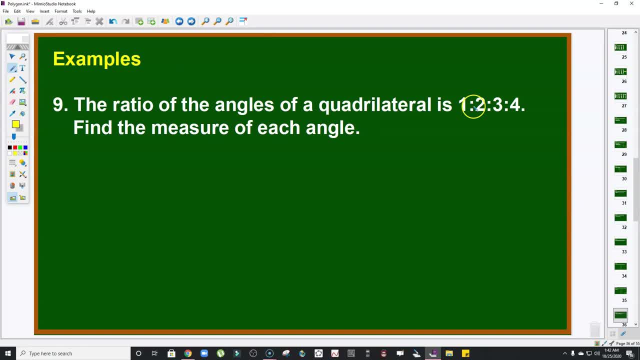 Find the measure of each angle. Again, ratio of the angles of a quadrilateral is 1 is to 2, is to 3, is to 4.. Okay, Any quadrilateral. Okay, So we know. Okay, If doing ko siyang x. 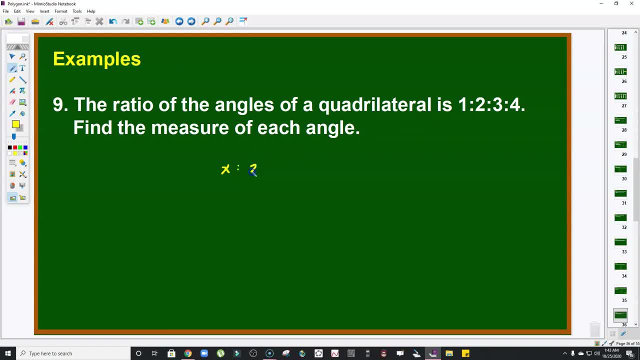 Alright, Tapos 2x, Hindi sinabing 1,, 2,, 3,, 4.. Basta x, Ah. 1 is to 2 is to 3 is to 4.. So I'll just use x here. 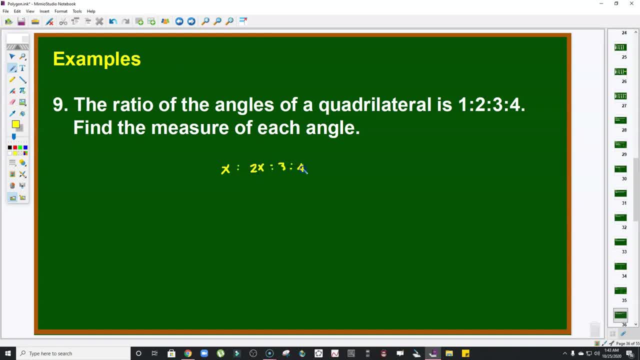 Okay, Parang ganda lalabas Right. Okay, Okay, Okay, Parang ganda lalabas Right. So since okay quadrilateral, the sum of each angle, the sum of the angle is 360.. 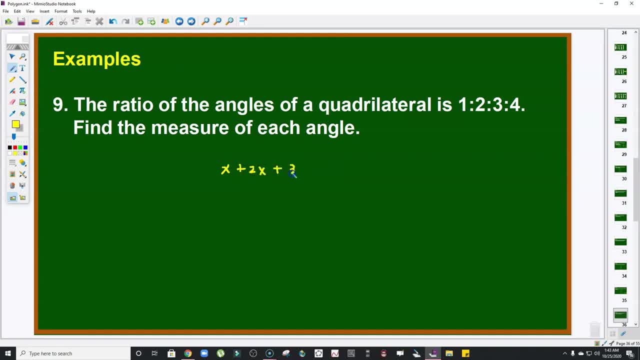 So therefore, I'll just add it: X plus 2x plus 3x plus 4x, that's equal to 360.. And we know, 1 plus 2 plus 3 plus 4, that is 10x. 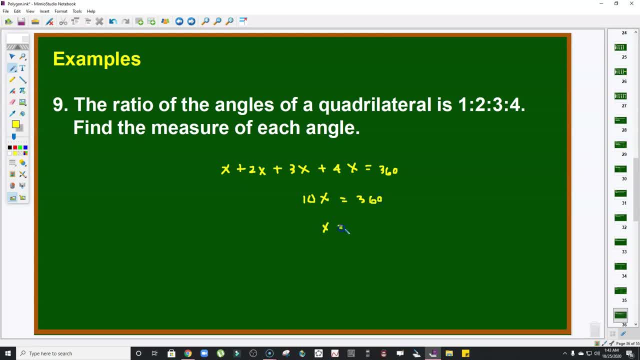 Right. So therefore, clearly, x is equal to 360.. Now tanong: Find the measure of each angle. So therefore, the measure of each angle are 60.. Ah, no, no, no, 60 tuloy. 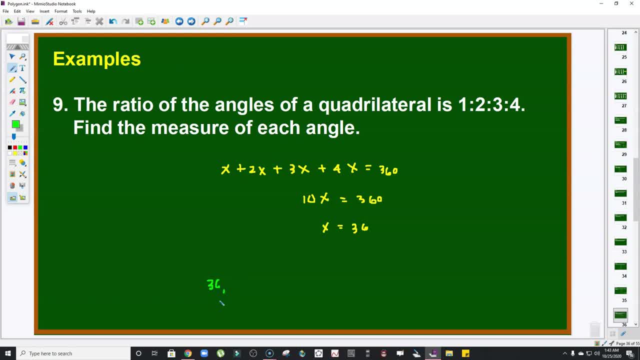 Sihan galing: 60.. Sorry, 36.. Tapos, 36 times 2, that's 72.. 36 times 3, that's 108.. And lastly, 36 times 4, that is 144.. 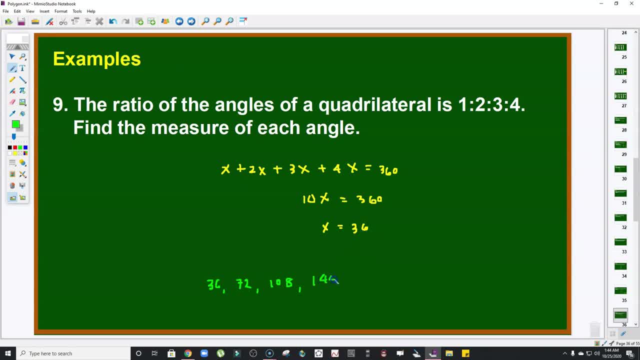 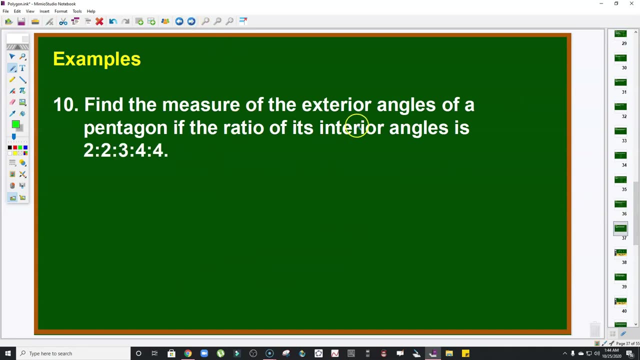 Right, 144.. So therefore, this is the measure of each angle. okay, Alright. last problem: okay for this video. Find the measure of the exterior angles of a pentagon. if the ratio of each interior angle is 2, is to 2, is to 3, is to 4, is to 4.. 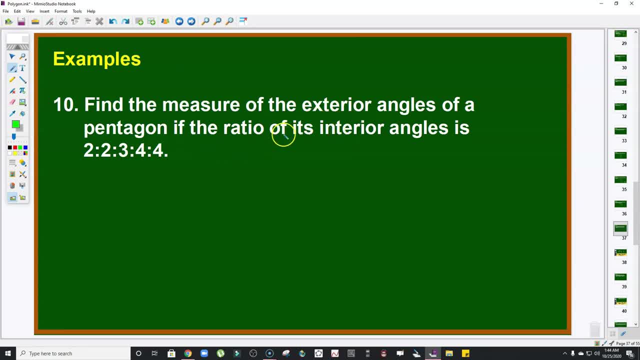 Again, what we're looking for is the exterior angle, okay, Okay. however, ang given yung measure ng interior angle is 2, is to 2, is to 3, is to 4, is to 4.. So, like what we did earlier, okay, 2x plus 2x plus 3x plus 4x plus 4x, equate natin kay 540, okay. 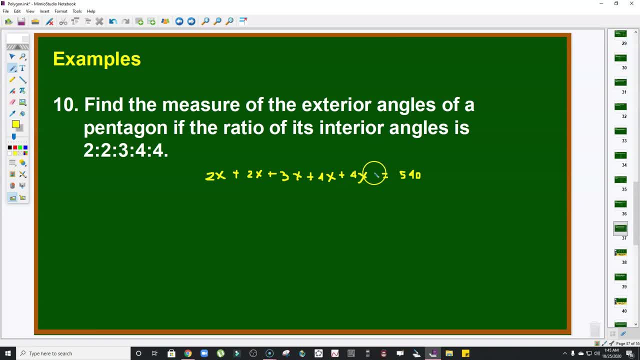 Because the measure ng angle sa pentagon is 540, see that Okay. so therefore ang 240.. 2 plus 2 plus 3 plus 4 plus 4, that's 15x. See that 15x equals 540. 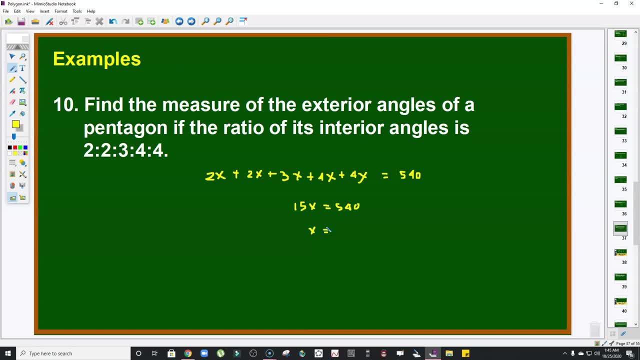 So therefore, 540, okay, 540 divided by 15, that is 36.. Okay, meaning to say yung measure ng: okay, ito yung interior angle. okay, Ito yung exterior angle. Take note, we're looking for the exterior angle. 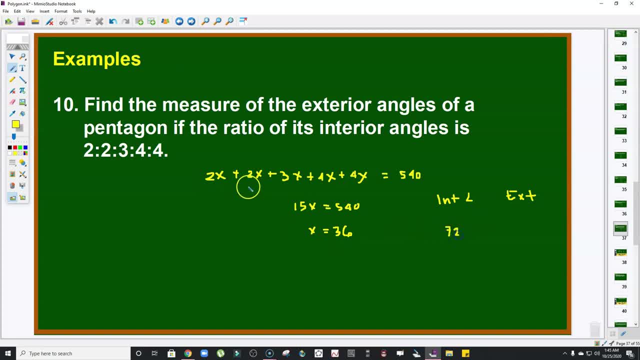 Yung interior angle: 36 times 2 is 72,. okay, Same yan 72 din. Okay. 36 times 3, that's 108.. 36 times 4, that's 144,, okay, 144.. 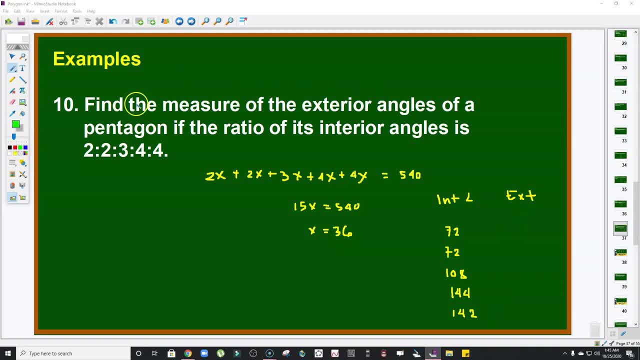 There you go. However, once again we're looking for the measure of the exterior angles. Okay, so syempre we know kapag exterior angle di ba. Okay, kunyari ito yung polygon ko Ayan. 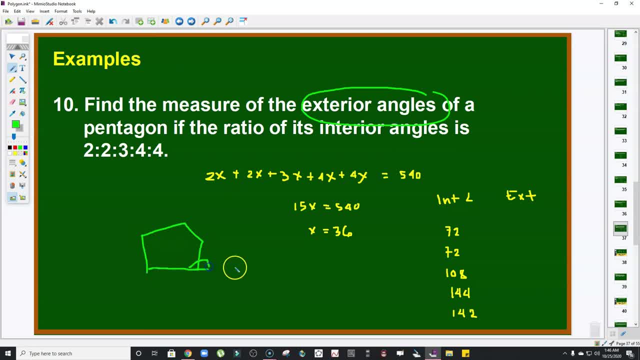 Pentagon ayan So ito linear pair Di ba linear pair yan. There you go. Okay so, all right. this is 144,. what happened? Sorry about that. Okay so, therefore, this is 108, okay, 108,. this is 72,, this is 36, and this is 36.. 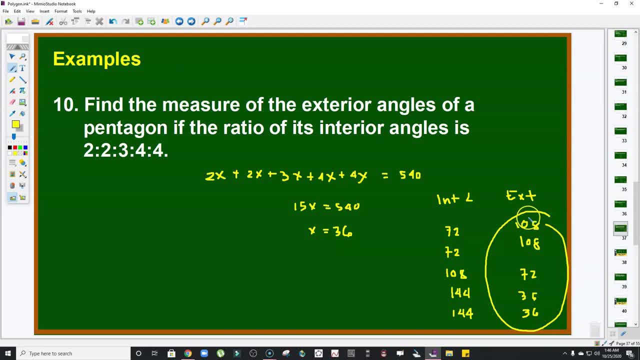 So if we're going to add all this 5,, the sum is 360.. There you go, Okay, so I hope you learned. I hope you learned something on this video, so feel free to share it to your batchmate. Keep safe.